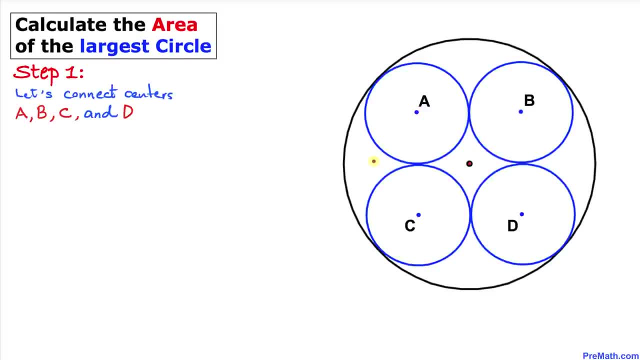 uppercase R. and here's our very first step. let's go ahead and connect these centers: a, B, C and D. let me go ahead and connect these one as you can see this: a B and then a C, and then C D and then B D. and here's our much nicer looking a. 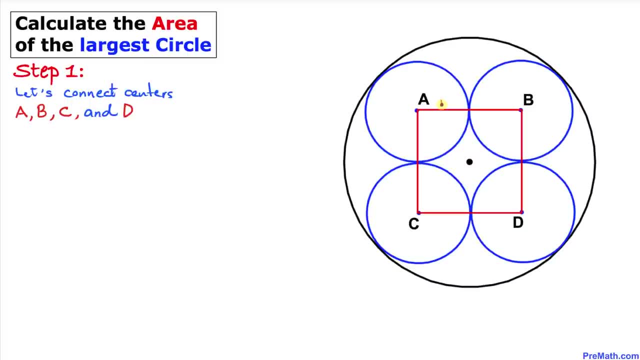 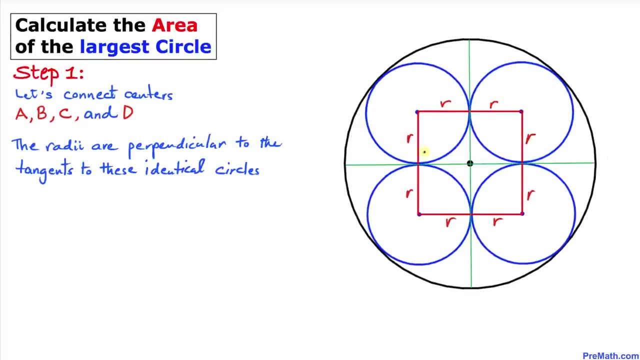 diagram and, as you can see, this one is our radius, lowercase R for these identical circles, R, likewise R, R, lowercase R, all the way, as you can see. and now we can go ahead and connect these centers, a, B and then a C, and then we can see that the radii of these identical circles are perpendicular to. 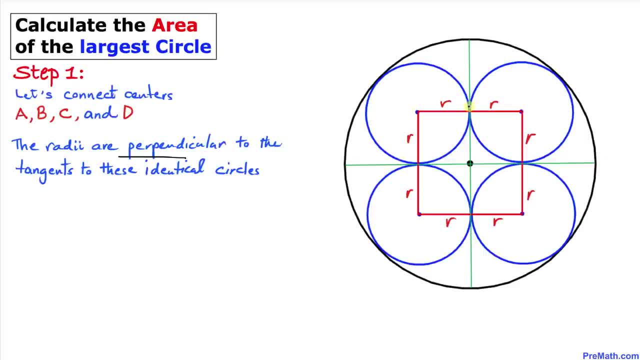 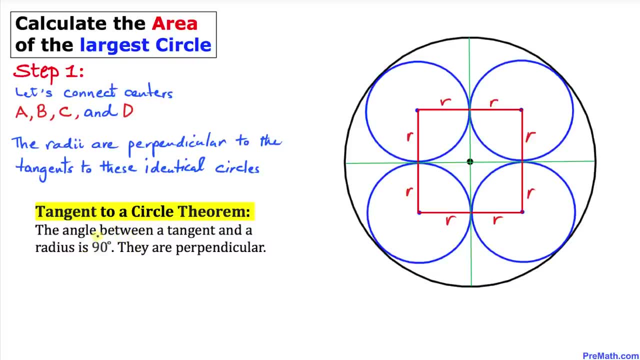 the tangents. as you can see in this figure- and here it's a tangent to a circle theorem- the angle between a tangent and radius is always 90 degrees. that means they are perpendicular. so that means this radius and this tangent to this circle is going to be 90 degrees. okay, 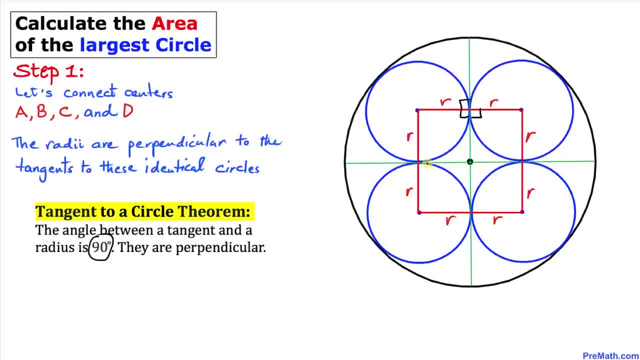 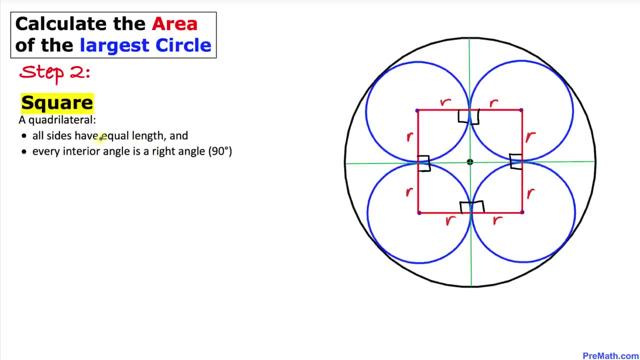 just keep in your mind: this is 90 degree as well. likewise, this is 90 degrees. this is 90 degrees. they are perpendicular to each other. according to this theorem- and now let's recall the square definition- all sides of a square have equal lengths and every interior angle is a right angle. that means 90. 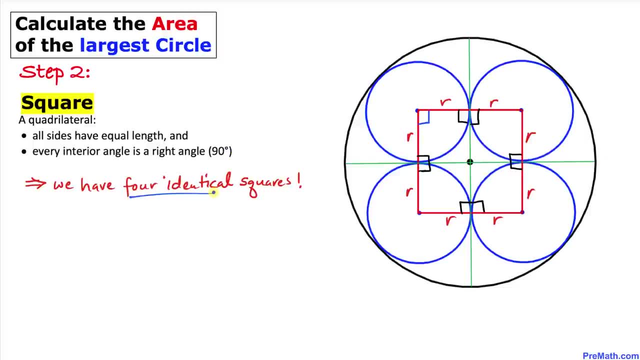 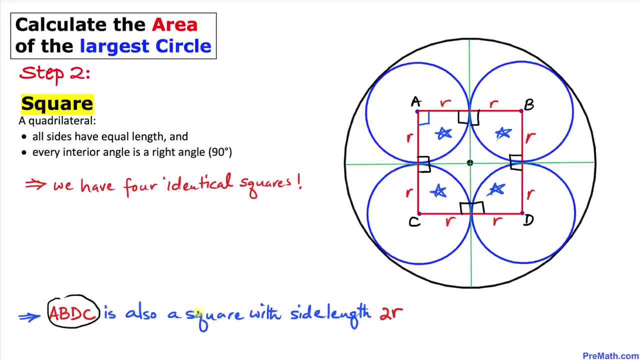 degrees, so therefore we have got four. I have identical squares as well this, this: they are all identical squares and therefore we conclude that this A, B, D, C is also a square, with the side length of this one is R and R. if we add these, one that is going to become 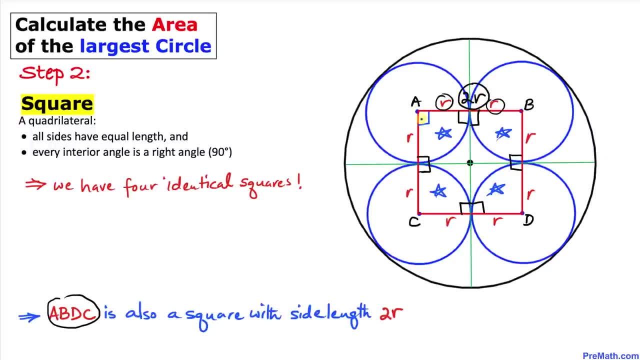 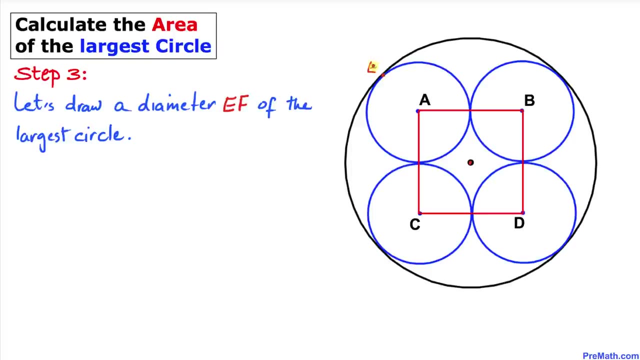 2, R. the side length of this square A, B, D, C- is going to be 2r. on this side as well, 2r and 2r, and here's our next step. let me go ahead and call this point e over here, this tangent and this tangent f, such that i am going to connect these points. 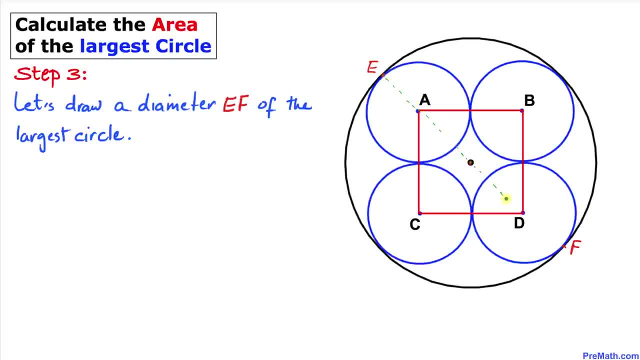 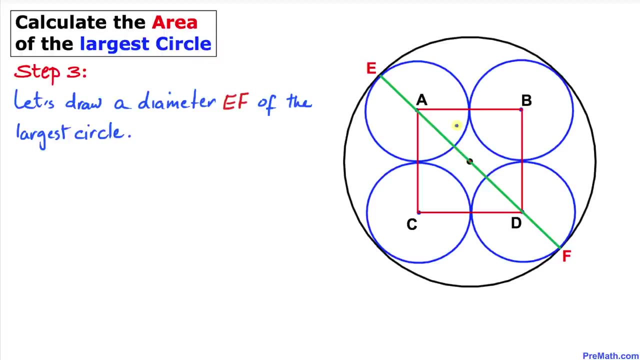 e and f very carefully, and this e and f is going to become the diameter of this largest circle, the bigger one. and here's our much nicer looking diagram. and now let's go in and observe one more thing. the main diagonal ad of this square, abdc, is a part of this diameter, ef. 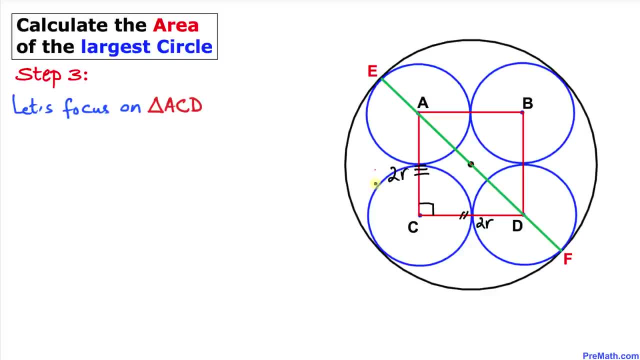 and now let's go ahead and call this point e over here, this tangent f, such that i am going to connect. now let's focus on this right triangle, acd. we know that this side is 2r and this side is 2r as well, so that means this triangle is an isosceles triangle, so therefore this is a special triangle. 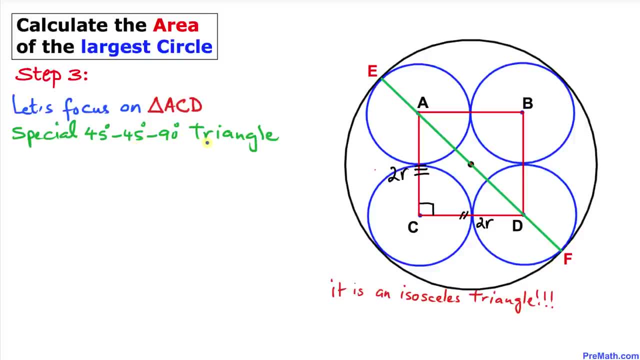 which is called 45- 45- 90 degree triangle. that means this angle is 90 degrees, this angle is 90 degrees and this angle is 90 degrees. and this angle is 90 degrees and this angle is 90 degrees angle is going to be 45 degrees and this angle is going to be 45 degrees as well. 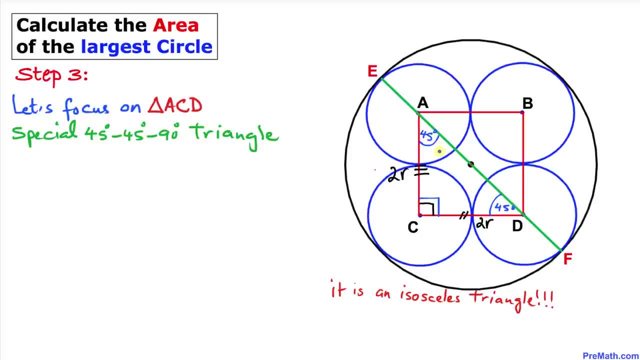 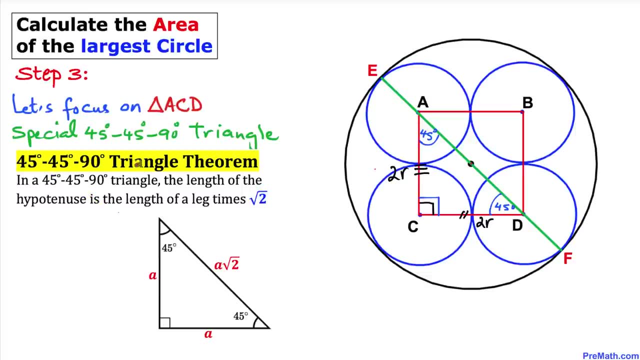 and if we add all these triangle we must have a 180 degrees. and here's our 45, 45, 90 degree triangle theorem. in a 45, 45, 90 degrees triangles, the length of the hypotenuse is the length of a leg times the square root of 2, as you can see over. 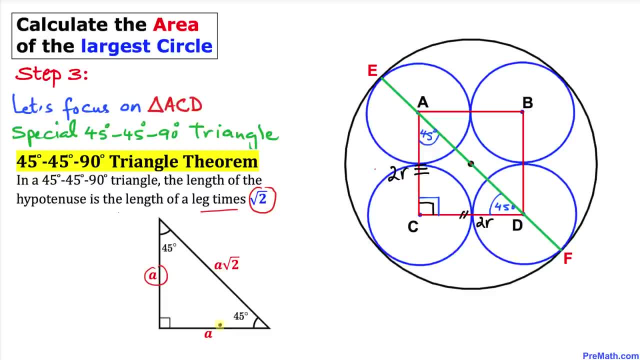 here. if our legs are a and a- over here they are same, then this hypotenuse is going to become a times square root of two and we are going to apply the same idea over here. in our case, if this is 2r and this is to r, then this side. 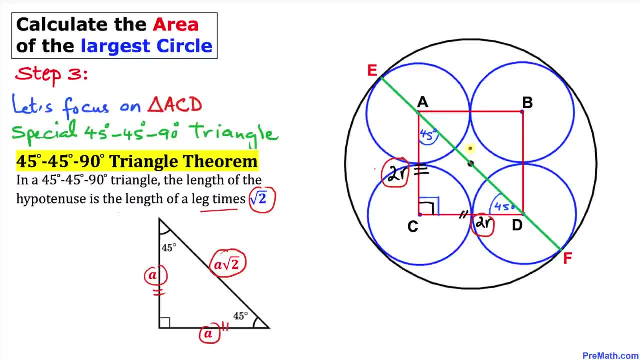 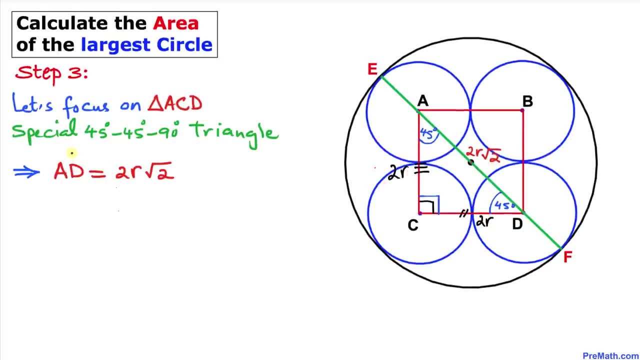 eight so far up top, this side a square, whatever. so now I am able to see that that side a squareır, or two quarter, is the length which is going to be lines. ad this, our hypotenuse is going to become simply 2r times square root of 2. so thus our length ad. 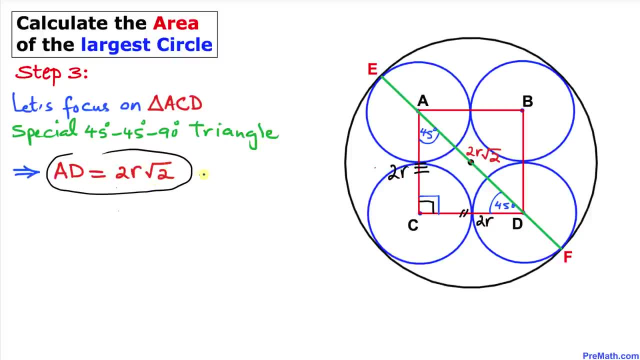 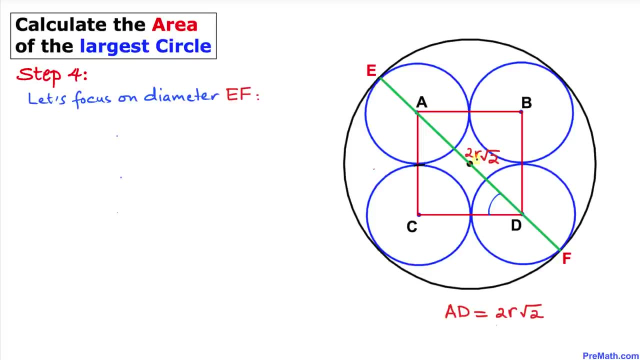 turns out to be 2r times square root of 2, and here's our next step. let's focus on this: our diameter ef. now we can see that this diameter ef is simply the sum of these line segments, ea, which is right here, and ea is nothing more than just the radius r, lowercase r r, all right. 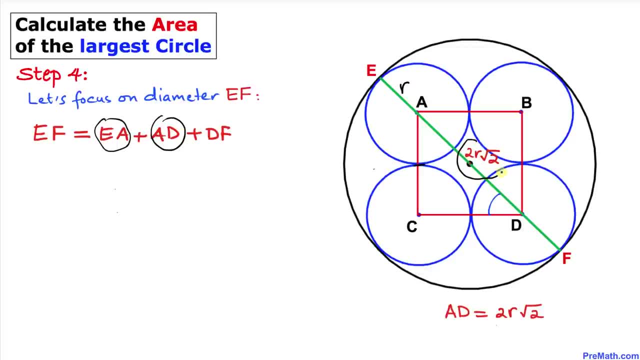 and ad is simply this: one 2r times square root of 2, and likewise this df is once again this radius, lowercase r. so let's go ahead and fill in the blanks so this become r plus 2r times square root of 2, and then plus r as well. so therefore, our ef value turns out to be simply. 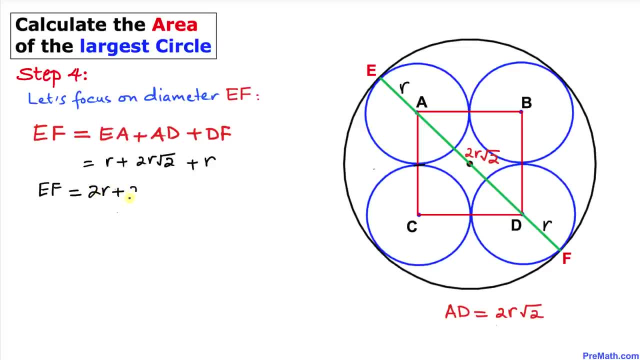 2r plus 2r times square root of 2, and i'm going to call this one as an equation number one. but also we know that the ef is a diameter of this largest circle. that means this radius is uppercase r and this radius is uppercase r as well. so that means diameter is. 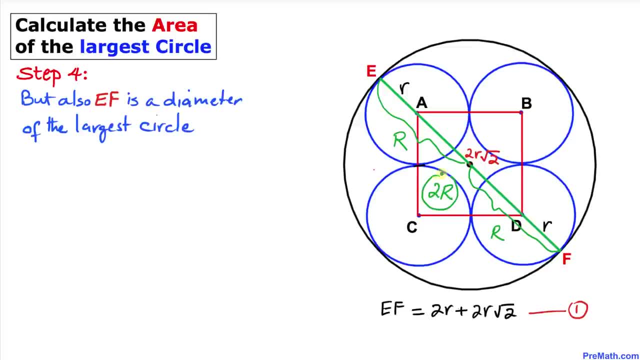 going to be simply r plus r is going to be 2 r. so therefore ef turns out to be two times uppercase r, and i'm going to call this equation number two. let's compare these equations one and two. here is our equation one, and here is our equation two, and then i'm going to. 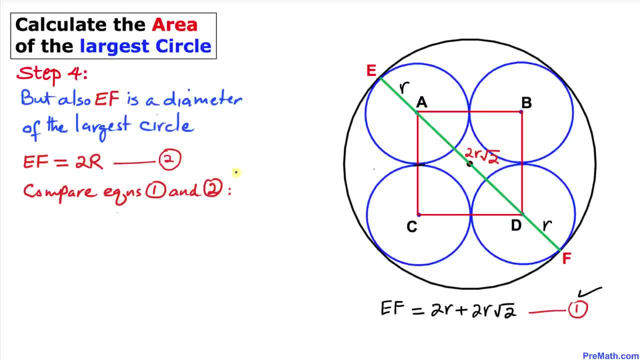 ca equation 2, so we can write them as: 2 times uppercase r equal to 2. lowercase r plus 2 r times square root of 2, and now I'm going to divide across the board by 2, as you can see, to make things simple. so we simply got r equal to lowercase r plus r times square root of 2.